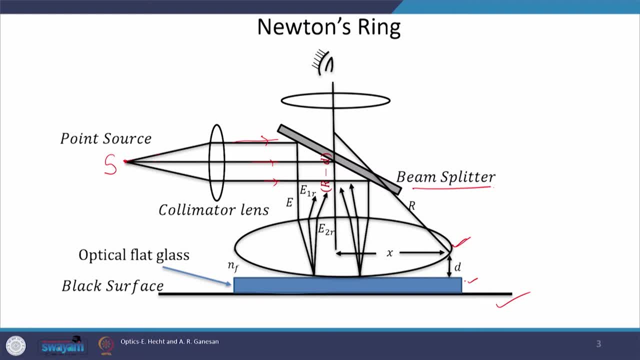 Now, this arrangement here is a lens kept on the top of a plain glass plate. okay, This is glass plate. Okay, and this is a flat glass plate and this is a convex lens. Now, when the beam falls normally on this system, then from the first interface, first surface, 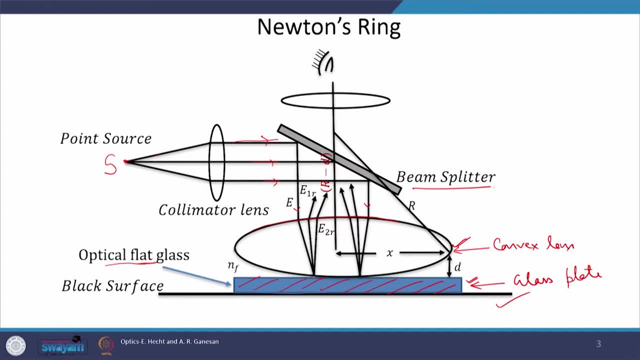 of the lens, the beam refract, Refract, Refract, Refract. So this is the second interface. Now, between the second interface, or lower interface of the lens and the top interface of the glass plate, there is an air film. yeah, Let us. 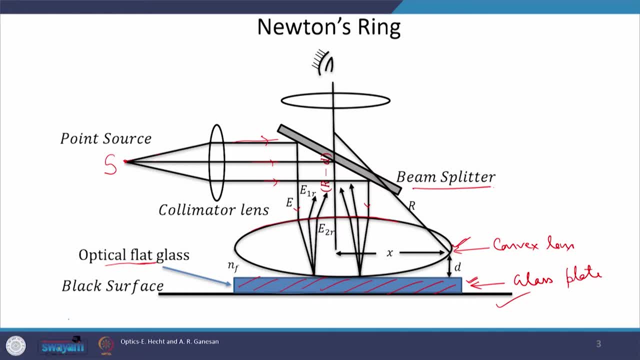 represent this air film with some colour. Let us pick this colour. This is the air film which is between the lens and the glass plate, the flat glass plate plate. Now, if you zoom in the area here, let us zoom in this part and after zooming it, 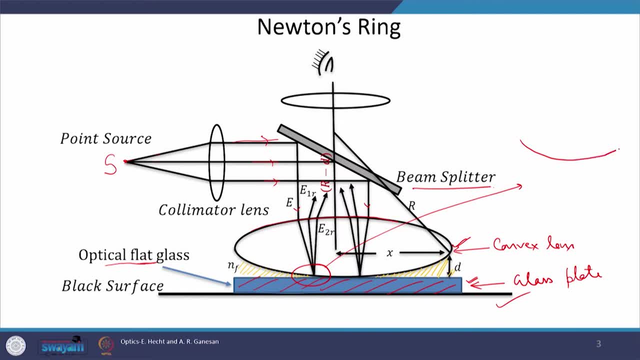 this is what you will see. this is the lens and this is your top interface of the glass, the flat glass. What happens is that the rays falls here and then it get reflected partially and transmitted partially, and the transmitted rays again get reflected partially up. 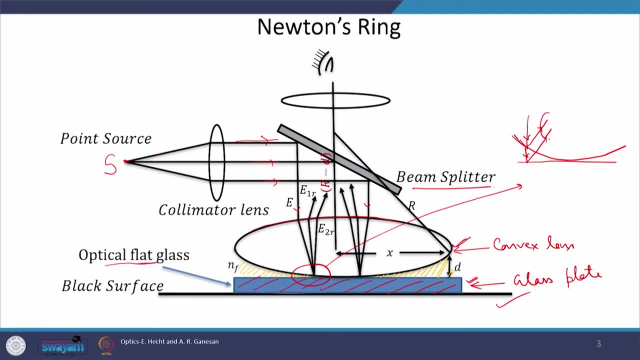 Now these rays, the reflected one, they interfere, these are parallel rays, and then we put lens and then they goes in our eyes And there we see the interference pattern. Now, due to the this air film, there is a part difference between the two reflected rays, and this is similar to the concept of wedge shape film. 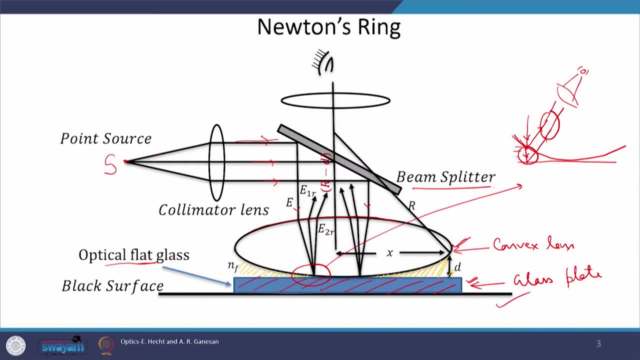 In wedge shape film we saw that two glass plates are oriented at some angle and this arrangement forms a wedge shape air film. Here the two lenses, the convex lens and this plain glass plate. it is forming a wedge, yeah, and in this wedge air is there and this air film now is responsible for the interference pattern. 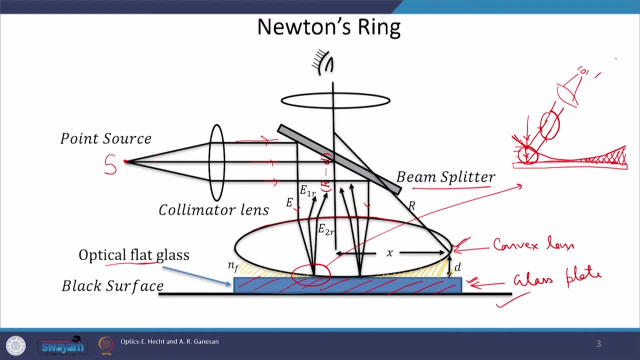 which we observe here in this Newton's ring experiment. Now suppose the incident ray has electric field amplitude e and the first reflected ray means this ray. it has amplitude n. So if this ray is very well-coordinated within the air film, it will not be able to produce the film. There is a very similar thing in 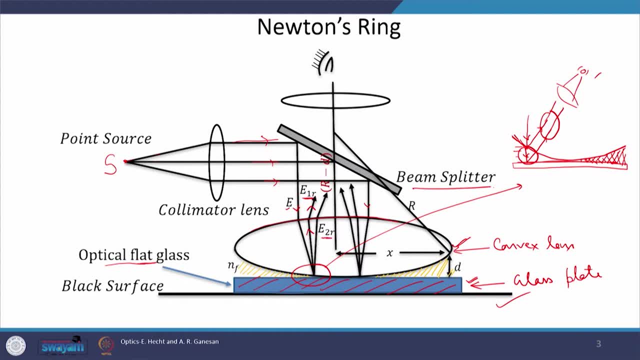 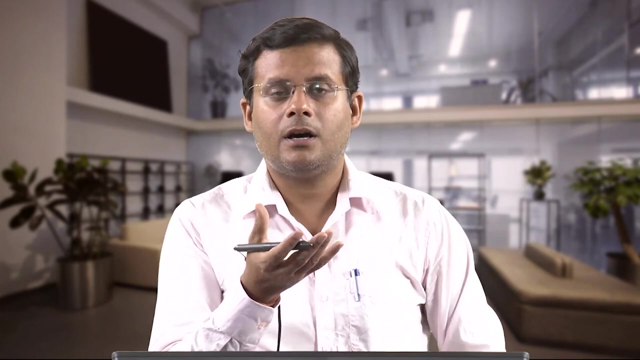 ray. it has amplitude E1r and the second reflected ray has amplitude E2r. Now this reflected beams E1r and E2r. they will interfere and produce interference fringes. Now we know that in 3D convex lens is a spherical structure or it has a circular symmetry. yeah, 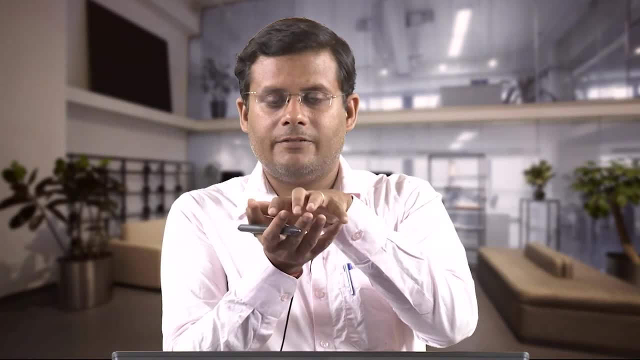 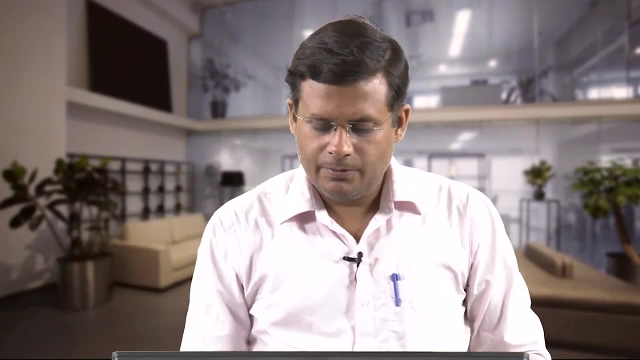 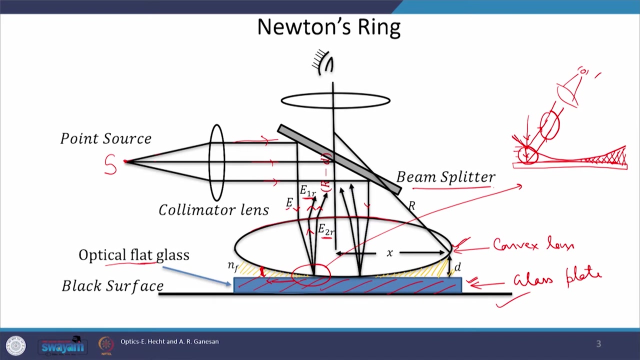 Convex lens is having a circular symmetry. it has a centre. around the centre there are symmetries. Now if we pick a certain air thickness here, then this air thickness, suppose, is at certain distance from the centre of this lens. then if we move around the lens with the same radius, 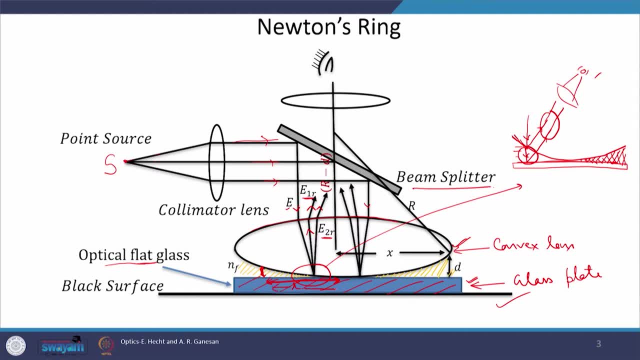 suppose this is our centre Small r radius, then the air film thickness would be the same. okay. If you view the same arrangement from the top, then you will see lens which is like this and a glass plate which is below the lens. okay, and if we pick a certain point, 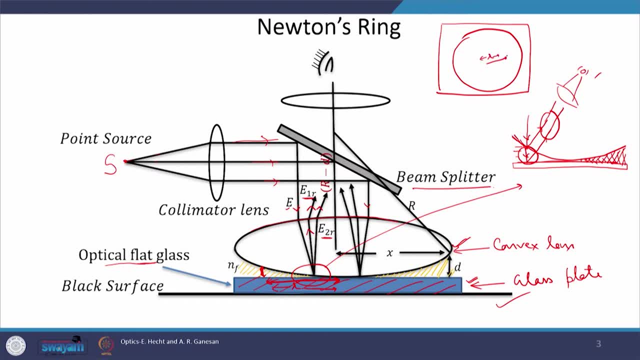 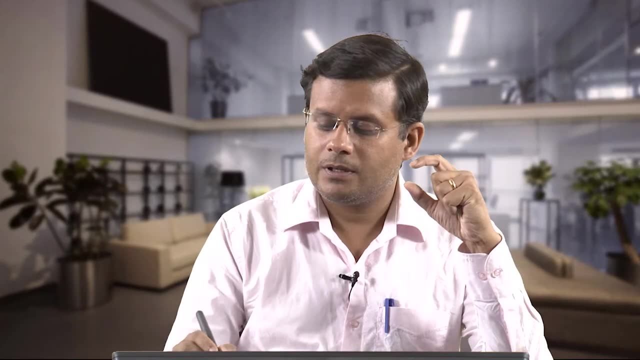 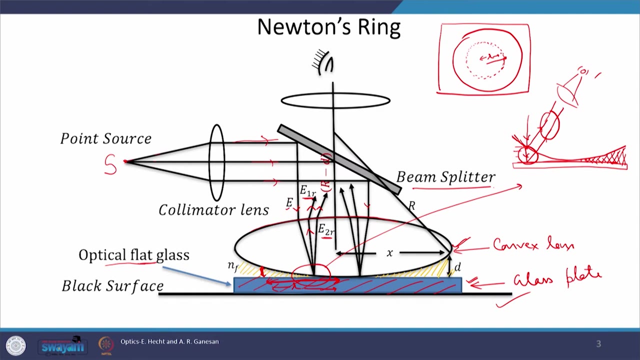 which is at r distance away from the centre of the lens. and then if you draw a circle of radius small r, Then the air gap, the thickness of the air gap between the glass plate and the lens, would be same on this circle. okay, and since the air gap is same on this circle, the condition: 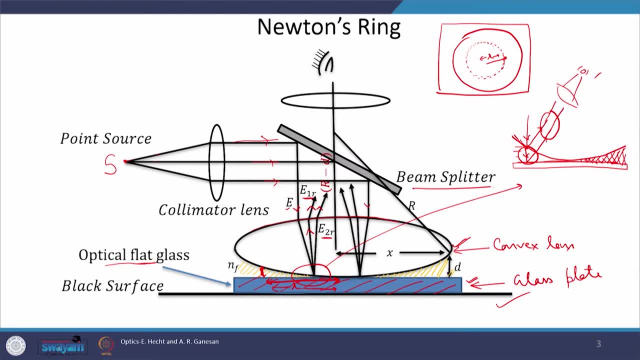 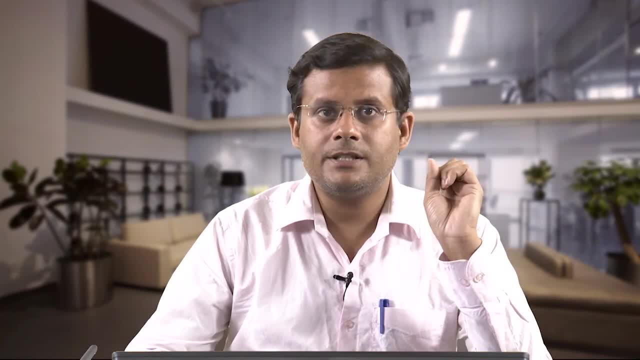 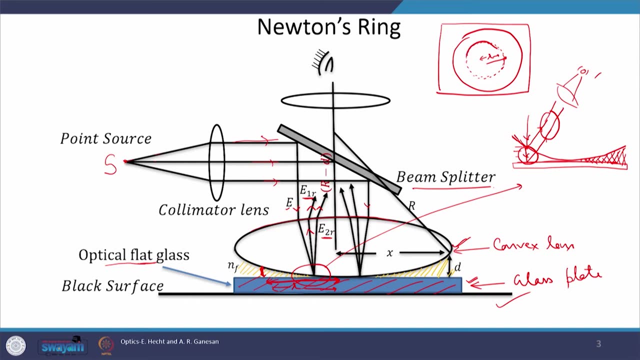 of maxima and minima or the type of fringe which is observed due to this air gap, will have the same intensity. What I mean by saying the same intensity is that if a bright ring is formed due to this air gap, then, or if bright colour is appearing, or if a dark colour is appearing due to this, 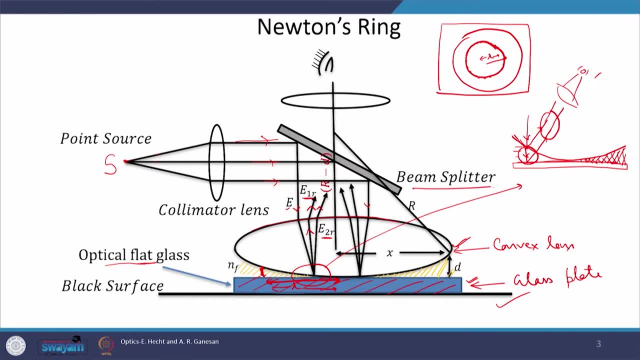 air gap, then this dark colour would be in form of circle, or the bright colour would be in form of circle around this centre of the lens. Therefore, the shape of the fringe- The fringe in Newton's ring experiment- will be circular. okay, we will observe concentric. 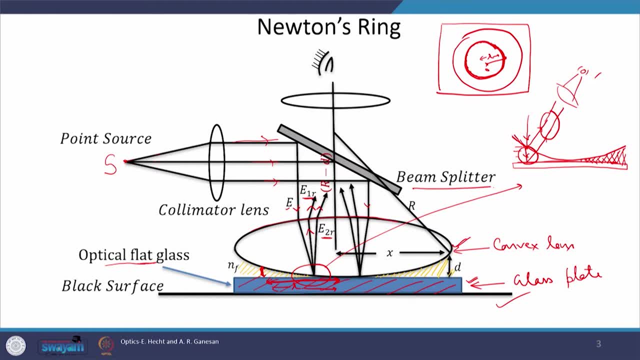 circular ring pattern in Newton's ring experiment. I repeat, Since there is a circular symmetry in this arrangement of air gap which is between the convex lens, lower surface of convex lens and upper surface of glass plate, this air gap will form a circle. 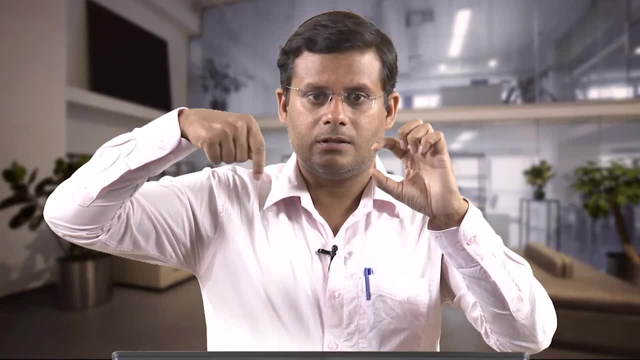 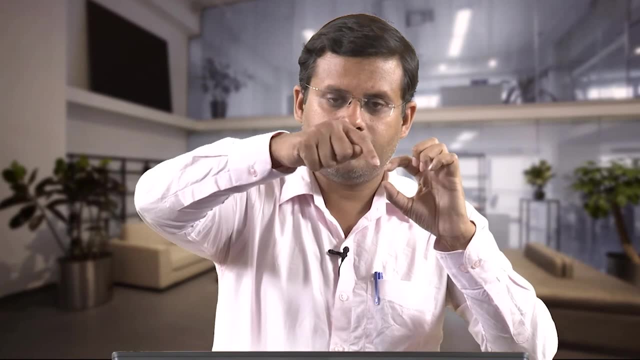 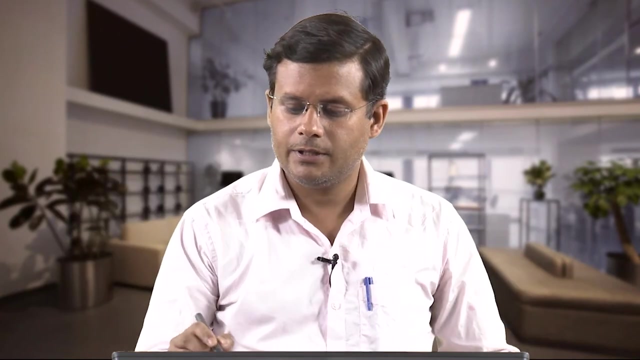 Okay, Okay, If we fix the height of the air gap, then we will find the same height of the air gap if we move around the centre of the lens on circle. okay, and this is what we are doing, This is the circle over which the air gap is constant. 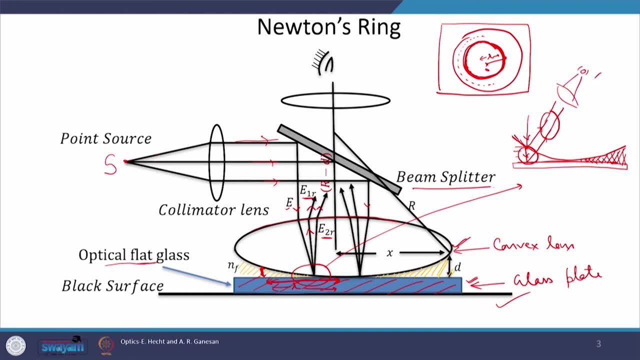 Similarly, you can again draw second circle, over which the width of the air gap would again be fixed Now, since the width of the air gap does not alter if we move on the periphery on the circumference of this circle. therefore, the intensity would be the same on this circle. 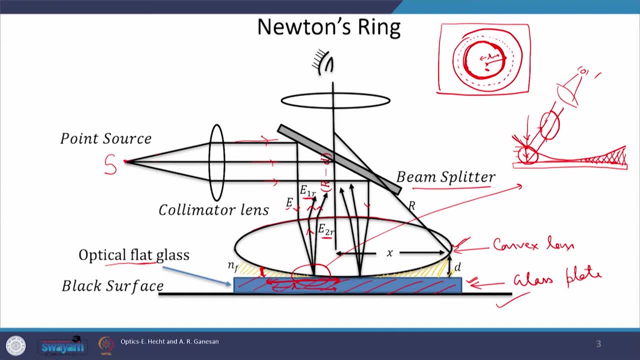 and therefore, if a dark pattern is seen on this circle, then it would be dark throughout, means at all point of the circle we will see dark, Okay, Okay. And if it is bright, then at all point of the circle, okay, on the periphery of the circle. 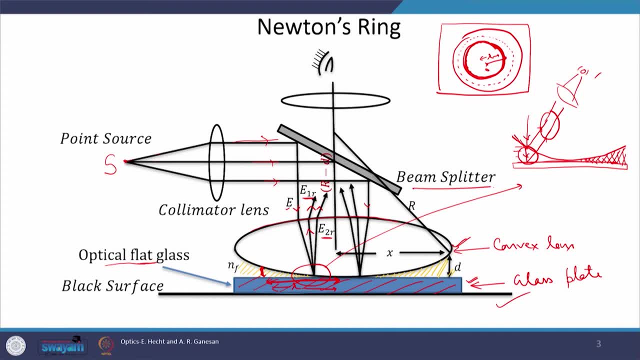 on the circumference of the circle, we will see bright. yeah, and therefore the fringe pattern in Newton's ring experiment, due to symmetry of the set up, is concentric circular. Okay, Now we see that as we move away from the centre of this system, this arrangement, the 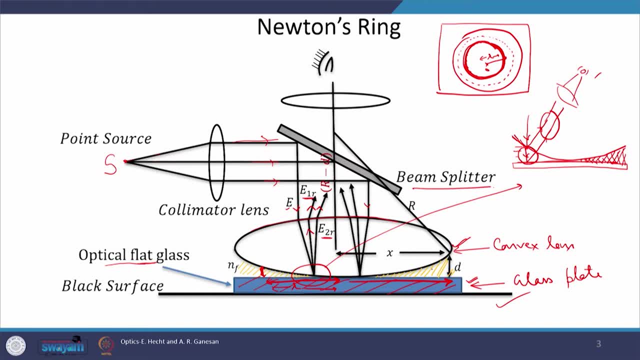 thickness of the air gap increases and therefore we may correlate this system from the wedge shape film which we studied in last class. Okay, Now suppose at certain point the air gap thickness is d, small d, which of course would be the function of x and x is the distance of this particular air gap from the centre. 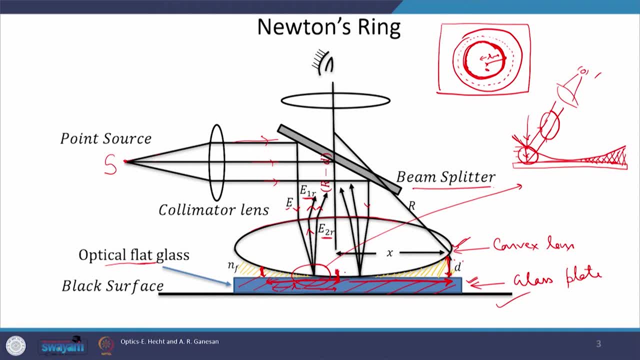 of the system. Okay, This is the centre of the lens. Okay, So the air gap, which is of d width, is at a distance, x, and we also assume that radius of curvature of the lens is r and we have drawn here the radius of curvature from this. 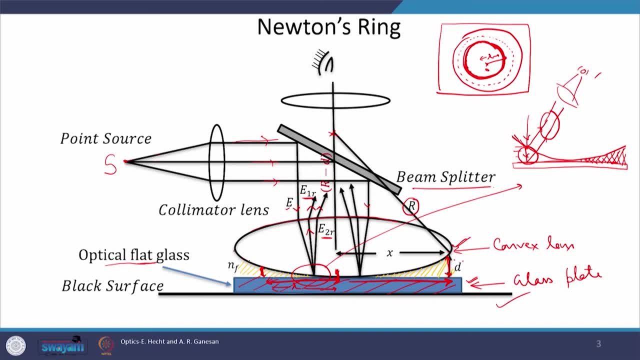 point, at the circumference to the centre of this lower interface here. If you draw a bigger circle here, then this bigger circle will have centre here and from here we have joined it. Okay, Okay, So from the distance, this would be capital R, which is the radius of curvature. 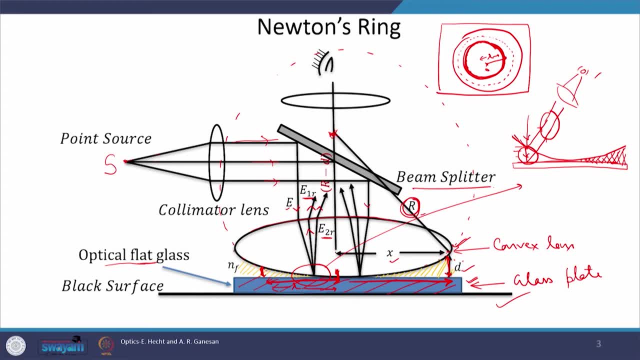 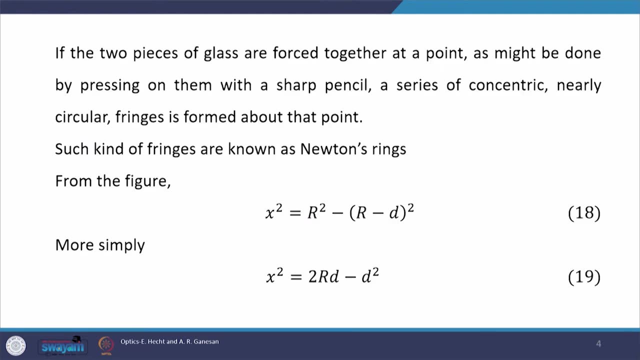 Okay, If d is given, x is known, r is known, then from the centre to the centre of the curvature, the distance would be r minus d. Yeah, This is the distance capital: R minus small d. Okay, Now from the figure, using Pythagoras: 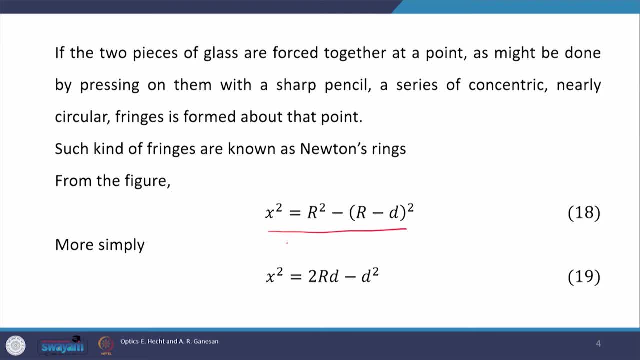 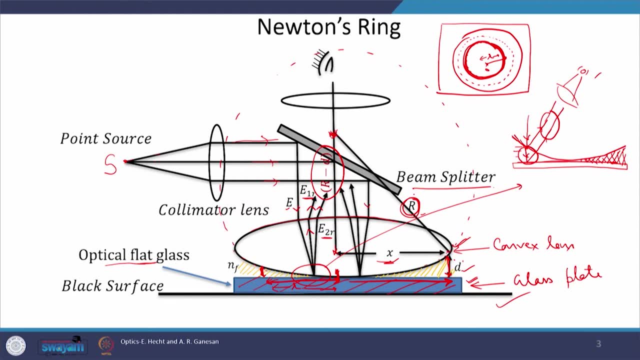 Okay, Pythagoras theorem: x square would be r square minus r, minus d whole square. yeah, You can see here in this figure x square, because r square would be from the Pythagoras theorem. r square would be x square plus r minus d whole square, and therefore from here. 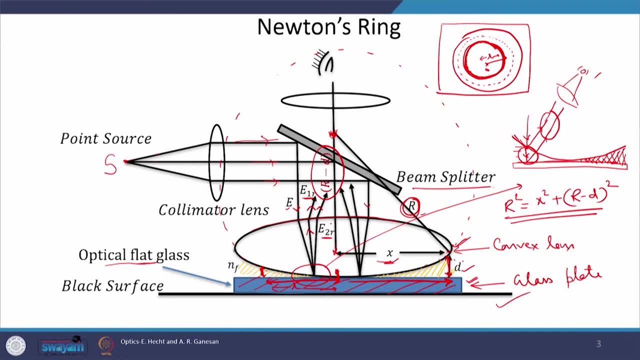 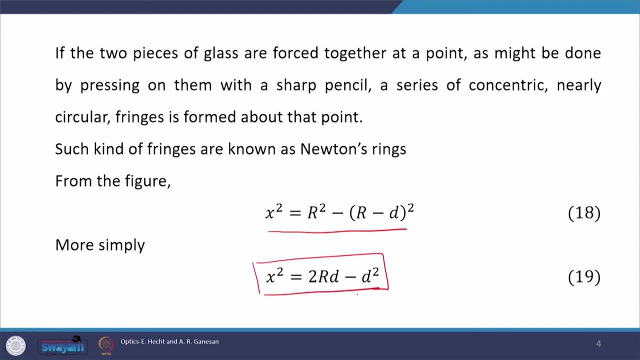 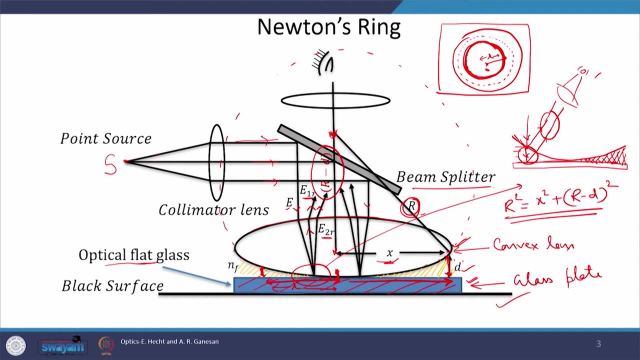 the expression of x would be: r square minus r minus d- whole square. Okay Now, if you expand it, then after simplification, we get this expression for x: square. Okay Now, since the radius of curvature, which is usually used in such setup, is very large as 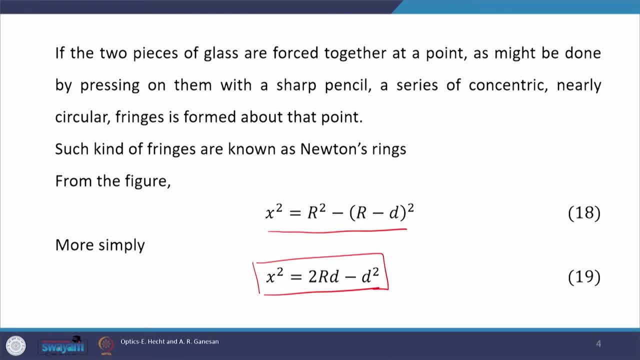 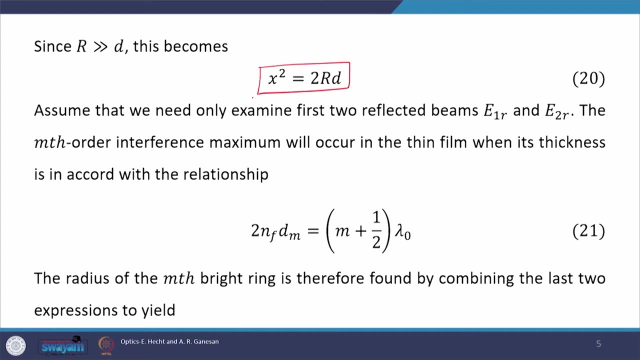 compared to the other distances involved. therefore, we can safely neglect the d square, because d is air gap, which is very small, relatively very small. Therefore, x square can be approximated to 2 r d. Okay Now, similar to what we did in wedge shape film, we are only considering two reflected 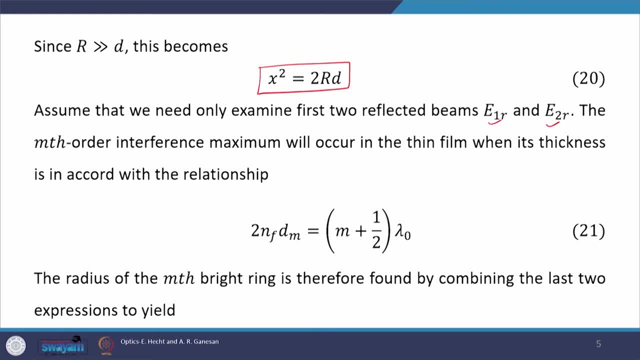 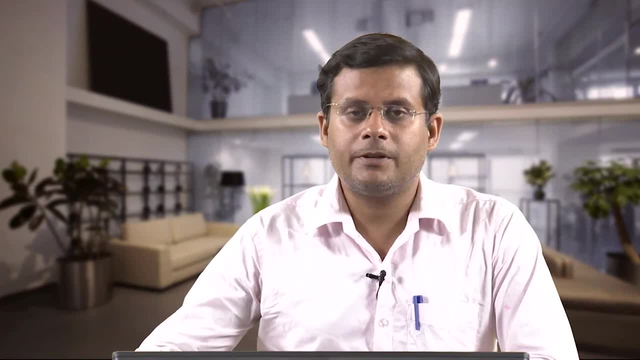 beams. Okay, First two reflected beams. Okay, Now, if we want to find the condition of maxima and minima, then we will again go back to our previous lecture, where we have already found the condition of maxima minima for. 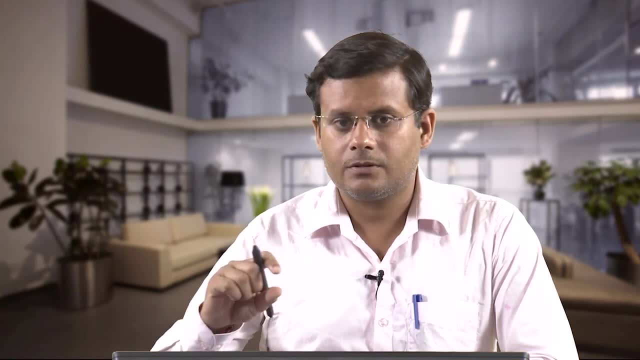 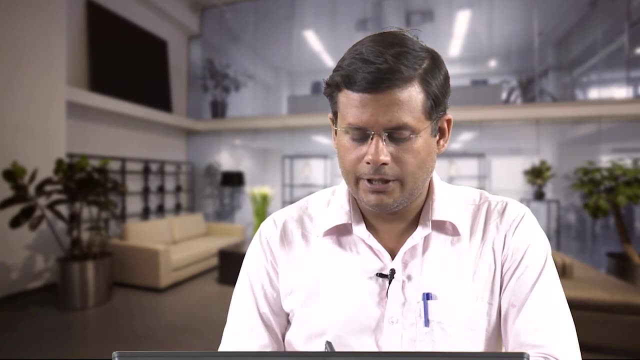 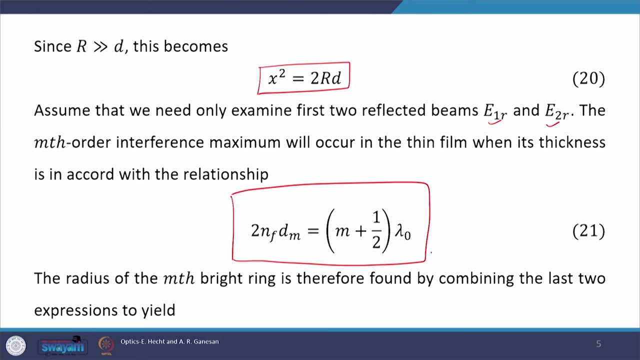 wedge shape film or for a glass plate of uniform thickness. thin glass plate, Okay. And from there we get this here. 2nfd is equal to m plus half lambda 0.. This is the condition of maxima, Okay. 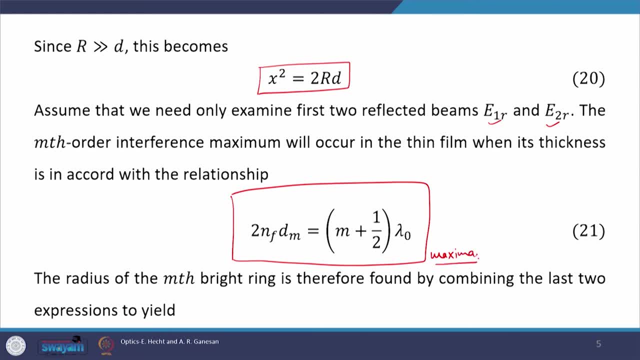 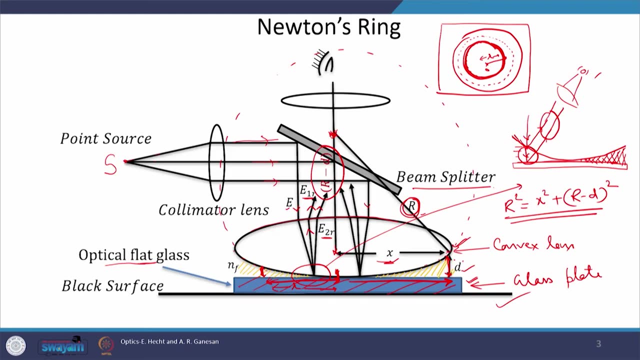 In reflection, of course. Okay, This we have already derived in case of thin glass plate. Okay, The point to be noted here is that cos theta term is absent from the left-hand side. Why is it absent? Because, from the figure, the incidence is almost at normal. 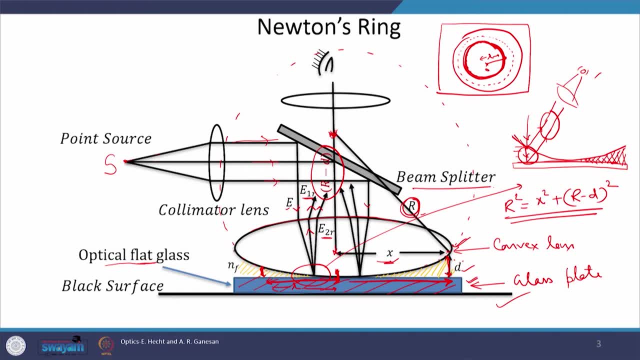 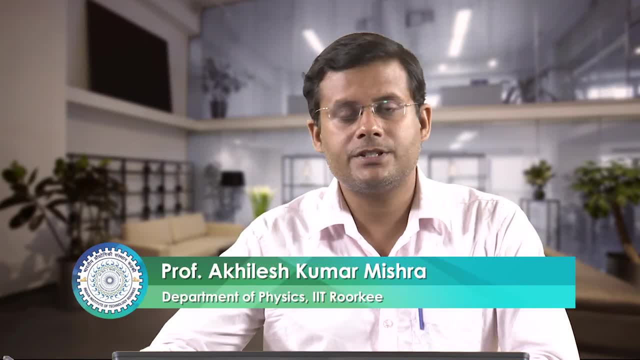 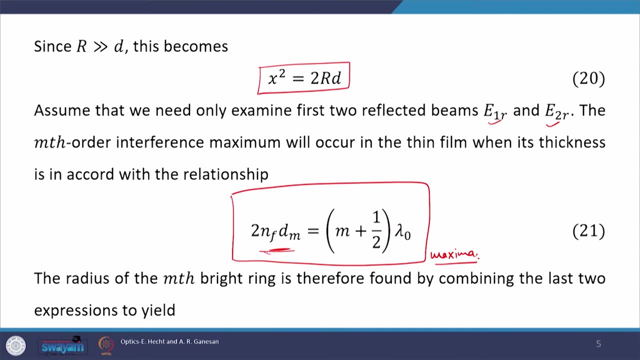 Okay, The incidence is almost normal And therefore the angle which our beam will make with the normal to the interface would be almost equal to 0. And therefore we can safely neglect cos theta term And therefore we do not have cos theta term here in this expression on the left-hand side. 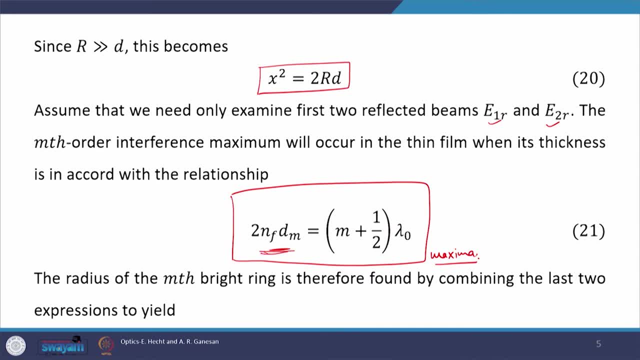 of equation 21,: 2nfdm only. Okay, Why 2?? Because the air thickness is being travelled twice by the second reflected beam. Okay, By Er2.. Okay, Now, this is a condition of maxima and therefore it should be integral multiple of lambda. but 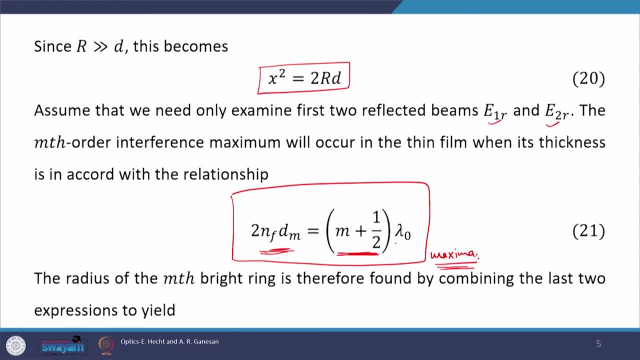 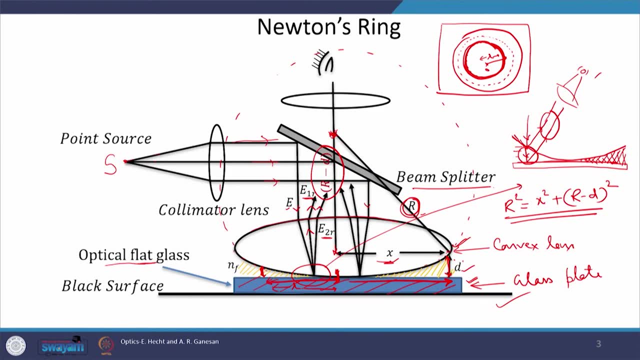 you are seeing, it is not integral multiple of lambda. Okay, There is something else. Why there is something extra? Okay, Because here in this figure, what you see is that suppose this is your interface, and then the light is coming in this direction, and then it is getting reflected here and 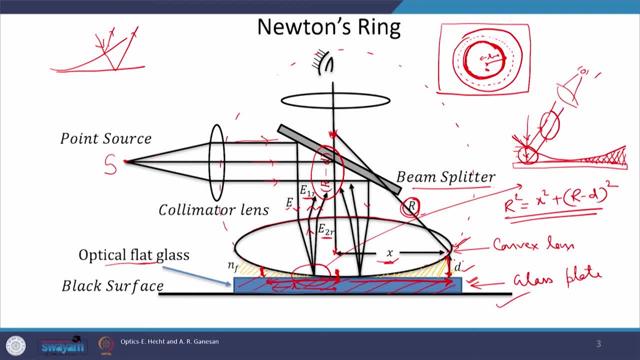 then it is coming here and then again it is getting reflected. Now, this first reflection, it is from denser medium to rarer medium, because this is air, this is glass and this is also glass. The first reflection is from denser medium to the rarer medium. 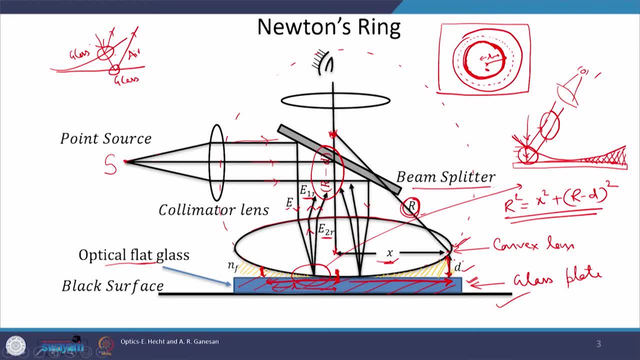 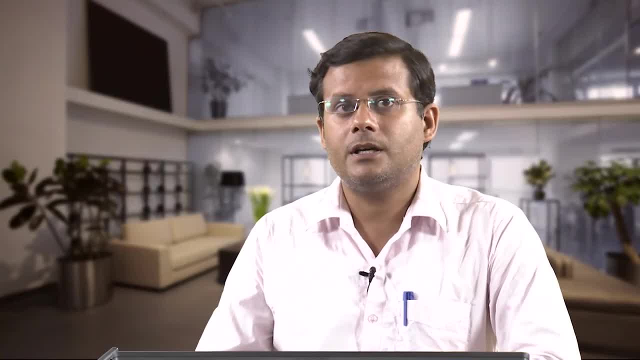 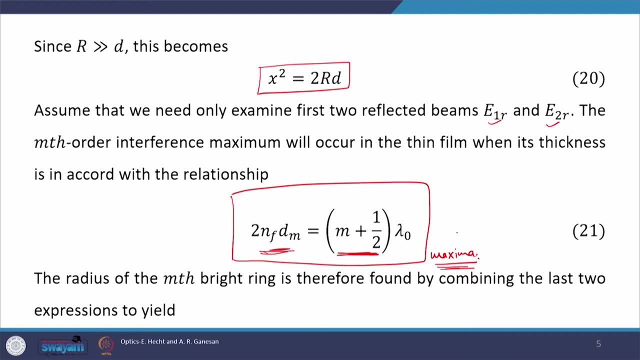 Okay, While the second reflection is from rarer medium to denser medium. Here too the extra phase difference of pi therefore appears and that, if you take into account, then the condition of minima now get converted into the condition of maxima, which is appearing here in form of equation 21.. 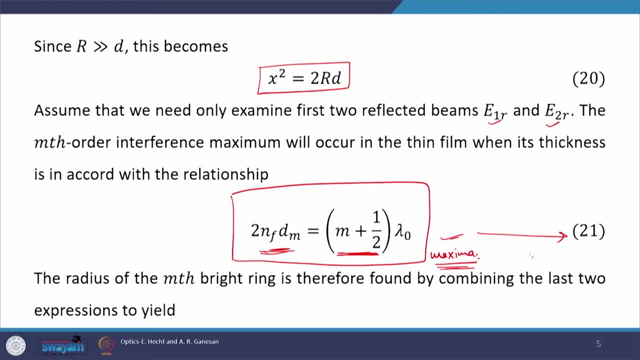 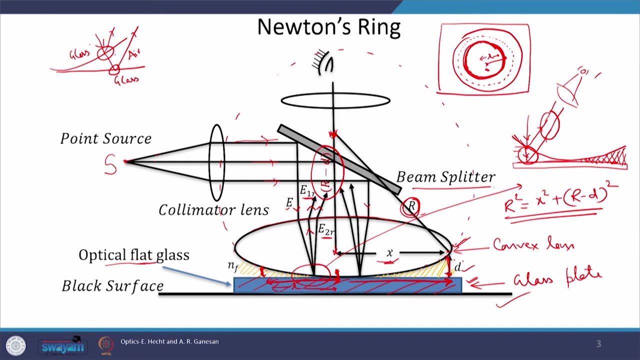 Okay, Now, if the condition of maxima is known, Okay, Then let us find out the radius of the mth bright ring. How to find out the radius of the mth bright ring? Let us go back to the figure, and we know the radius is expressed by small x and in this: 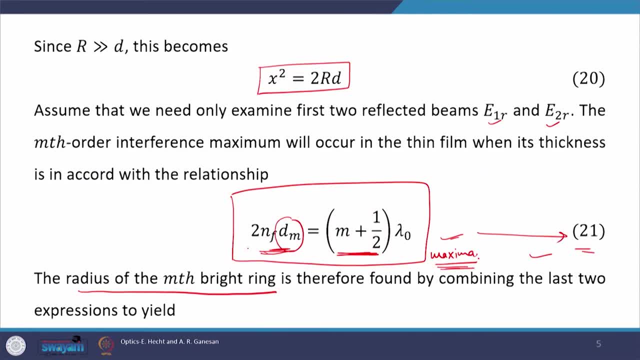 expression of 21,. we have d. How the d is related to x through equation 21?. We will substitute for d here. Then d would be equal to x square upon 2r. We will substitute Ah- This is the value of d- into equation number 21.. 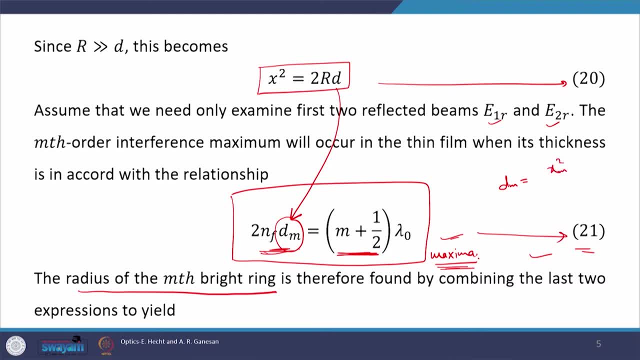 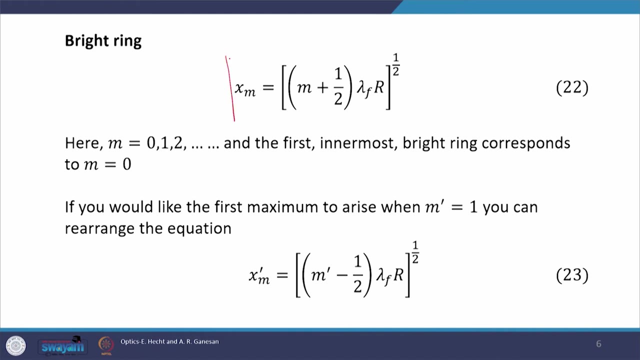 What is the value of d? dm would be xm square plus 2r capital R. I am associating subscript m with d and x just to indicate that these calculations are for mth bright ring. Okay, Now, if you do this substitution, then for the bright ring the value of the radius is: 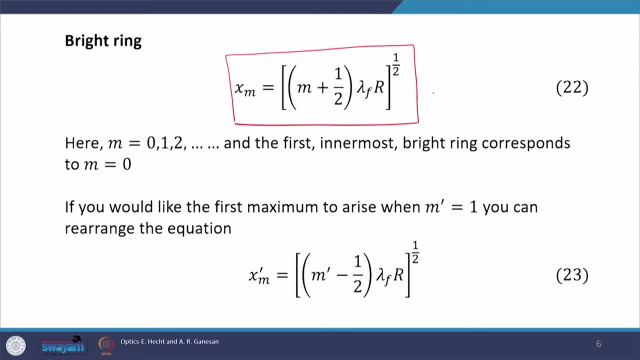 here, Yeah, And it is given by this expression, number 22, where m, of course, is an integer number. Okay, Now, the smallest value of m is equal to 0.. Okay, And therefore innermost bright ring correspond to m is equal to 0. 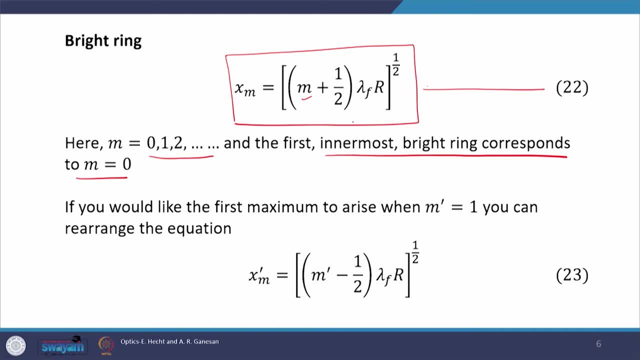 Okay, Now you can rearrange equation number 22.. Okay, And if, because we are talking about first bright ring, then sometimes people think that m should start from 1.. And if you want m to start from 1,, then the equation get modified slightly. 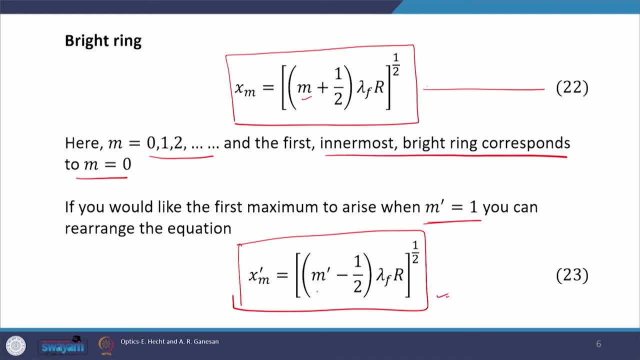 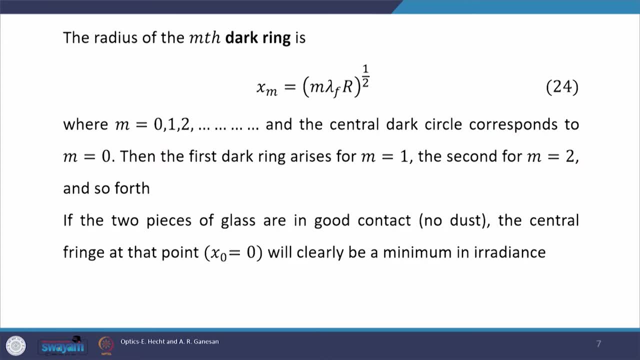 Okay, Then after rearrangement, equation 22 get converted into 23.. They are the same thing but written differently. Now, once the expression for R, expression for radius of mth bright ring is given, then the equation gets modified slightly. Okay. 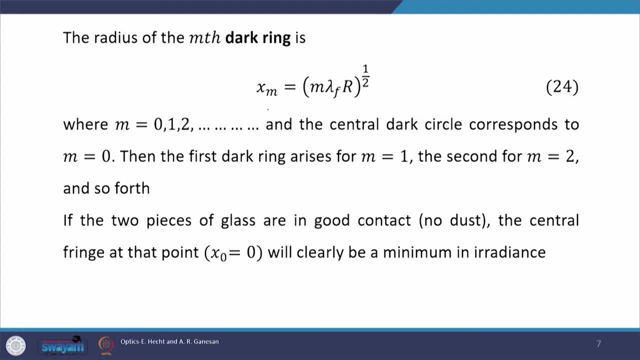 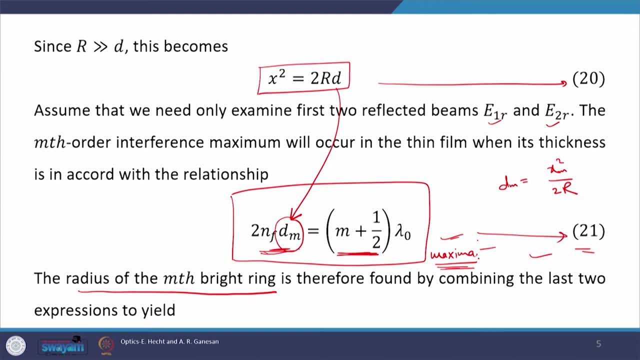 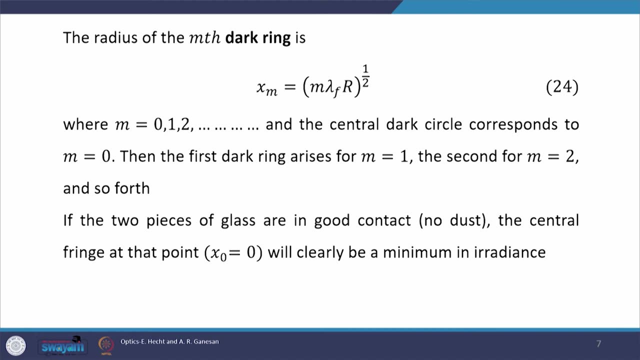 So here, bright ring is known, Let us find it for the dark ring. Now we will follow the same thing here. the condition of maxima is here. Similarly, we can get the condition of minima, Okay, And there, instead of odd integral multiple, we will result to integral multiple of wavelength. 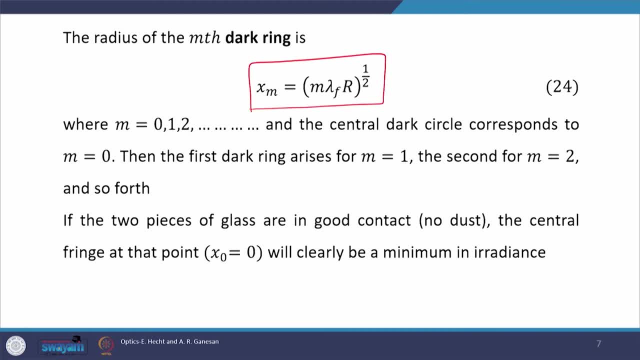 and from there we get this expression. This is the expression for radius of dark ring, mth dark ring. Here again, small m is an integer, Okay, And you can see that central dark circle or central dark pattern corresponds to m is equal to 0.. 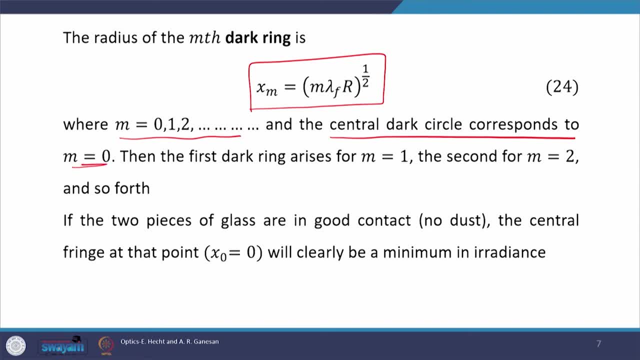 Okay, Because when m is equal to 0, xm is equal to 0, which obviously correspond to the central patch, central dark pattern. Okay, Then the first dark ring arises when m is equal to 1, for the second, we will have to. 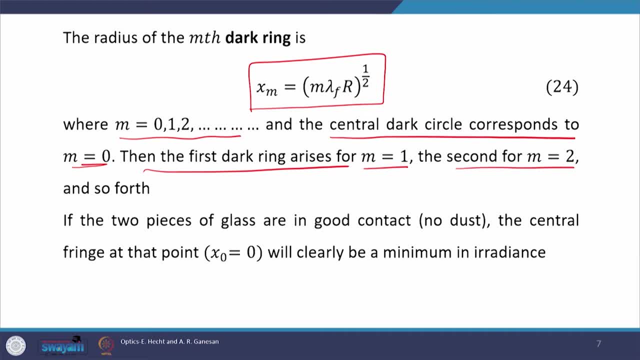 substitute: m is equal to 2.. Okay, Okay, Now again, this is the lower interface of the lens and this is the upper interface of the glass, the glass plate. Now you know, at for m is equal to 0, there is no thickness here. 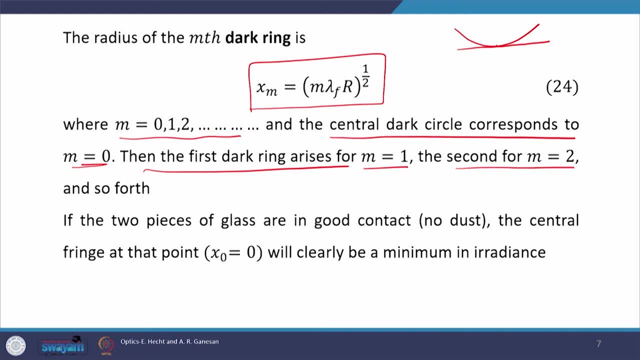 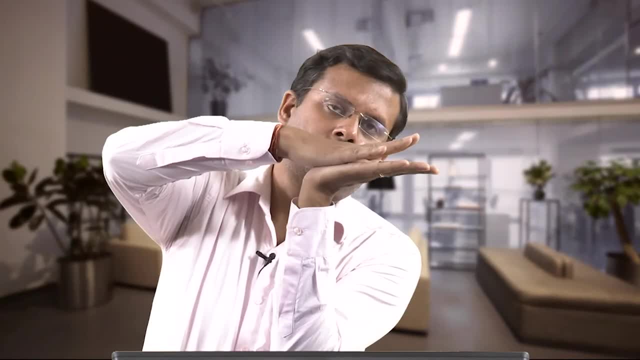 The glass plate is touching the convex surface of the lens. here, This is this type of arrangement: The glass plate is touching the lens. Okay, There is 0 air gap. Okay, If the air gap is 0.. Okay, Then the path length difference is also 0. 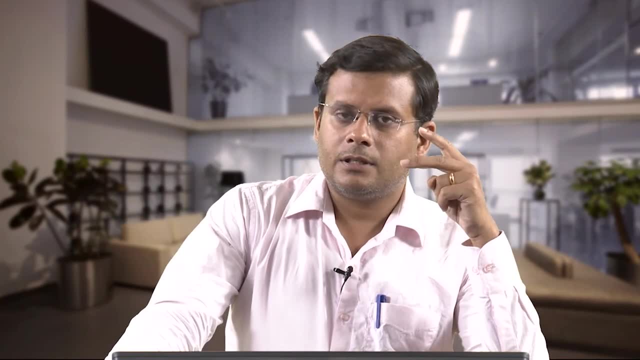 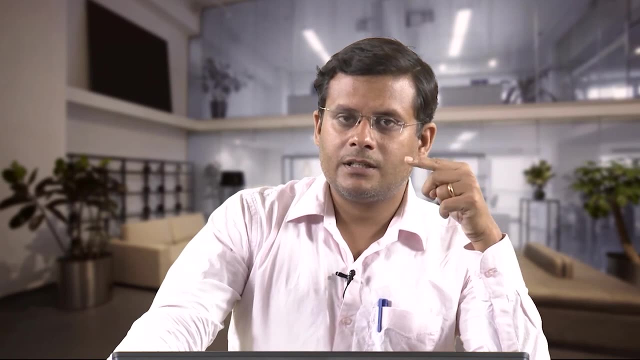 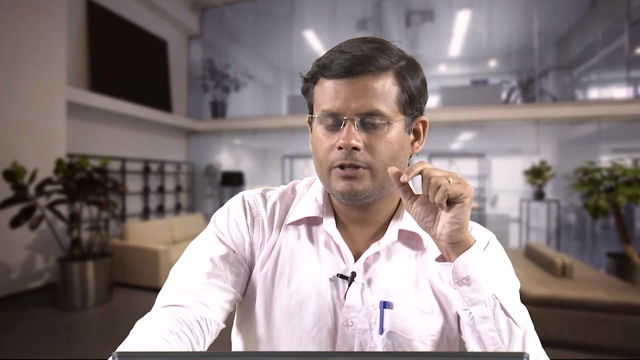 Okay, There are. the interference is happening between two, first two reflected beams. The first reflection is at the interface of lower surface of glass or lower surface of lens, and the second reflection is happening at the top surface of glass plate. These two reflections then interfere. 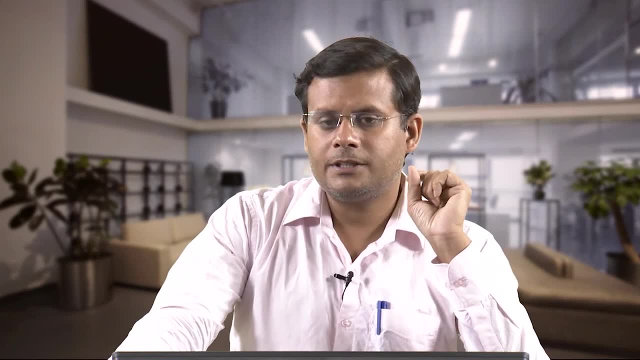 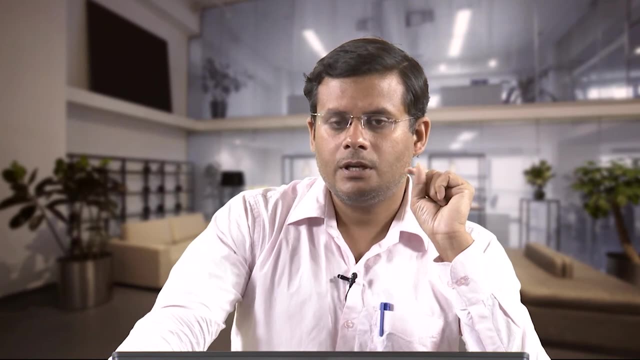 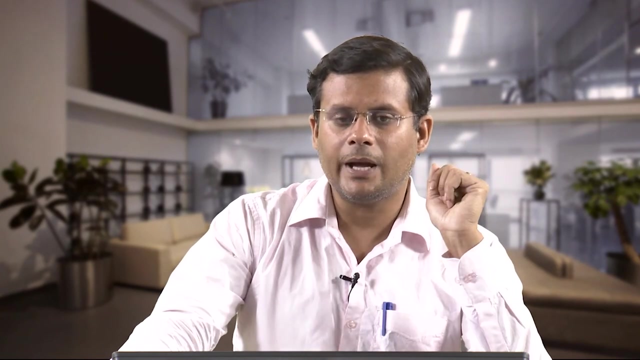 Okay, If the air gap between the two interfaces is 0,, then the path length difference between these two rays would be 0, and if the path length difference is 0,, then one can one quickly says that that it is the condition of maxima. 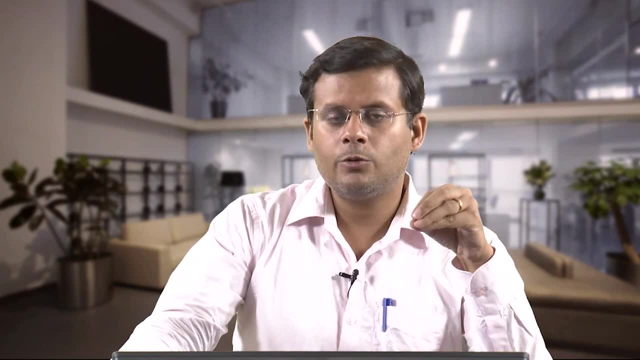 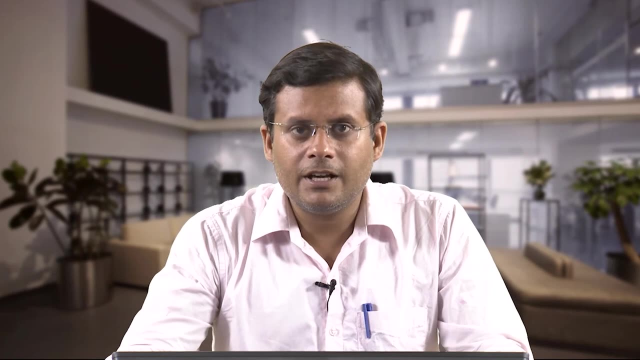 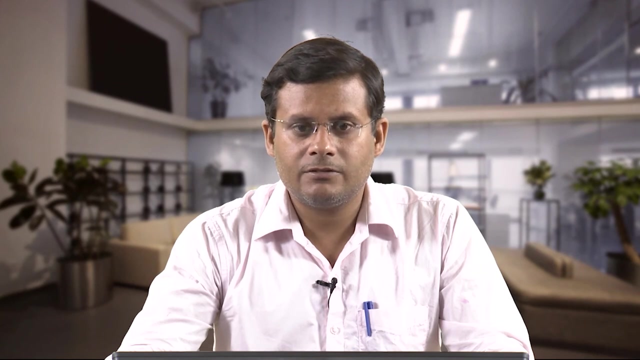 But before commenting this, before making such an statement, we must think about the internal and external reflections which are occurring here. In this case, yeah, In our case, the first reflection is from denser medium to rarer medium and the second reflection is from rarer medium to denser medium. 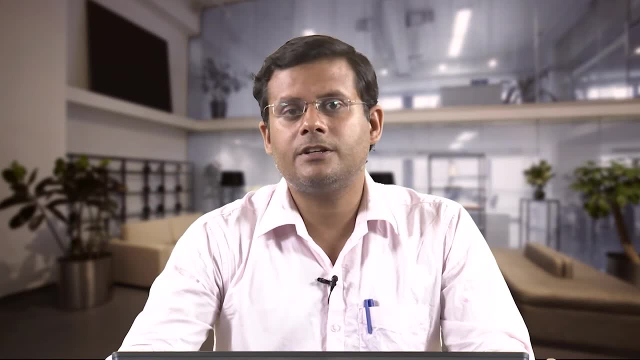 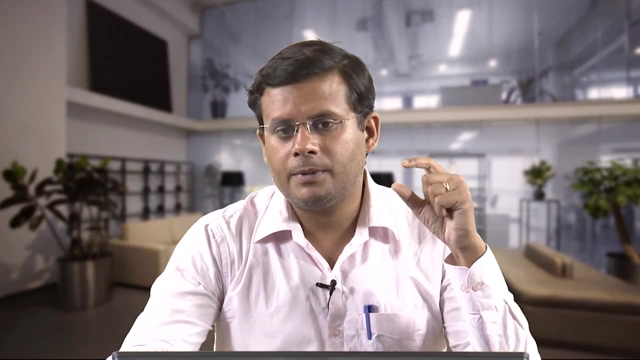 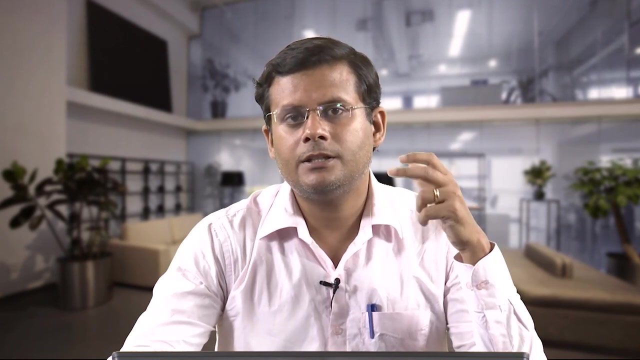 Therefore, we must take into account the extra phase difference, pi, which is creating due to these reflections and therefore, even if the optical path length difference is 0, due to reflection, the extra phase difference of pi is being introduced. Okay, And therefore the condition of maxima is the condition of minima and vice versa. 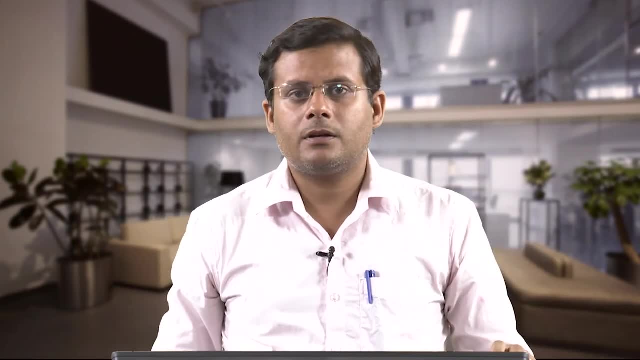 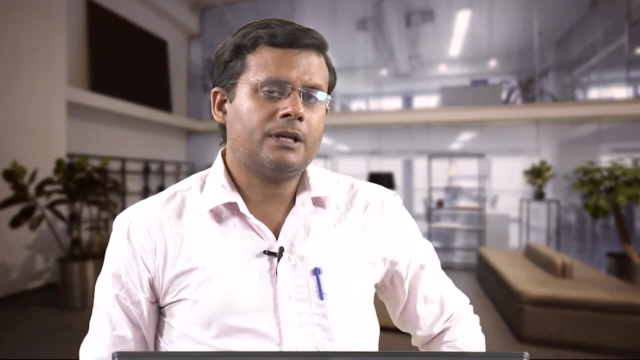 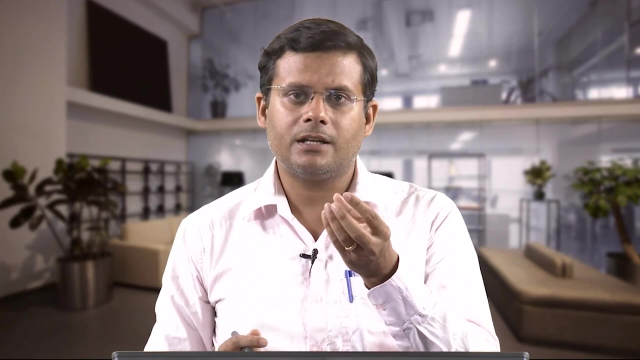 And therefore, even with 0 air gap, we get dark patch at the centre. Okay, But while performing the experiment- sometimes so happen- is that we do not see the dark pattern. People see bright there. This is because insertion of small dust particle. 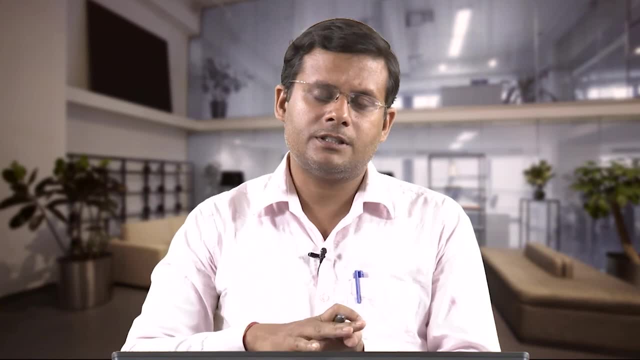 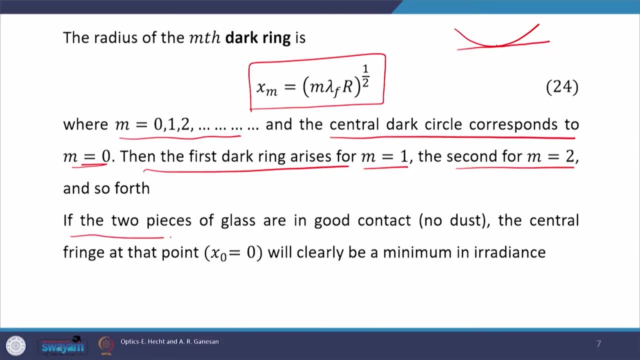 Okay, The two surfaces do not contact touches properly. Yeah, So few dust particles sit there and we see some bright patches there too. But if the two plates of two pieces of glass are in good contact- good contact means if there is no dust- then the central fringe at point x0 is equal to 0, x0 means for the 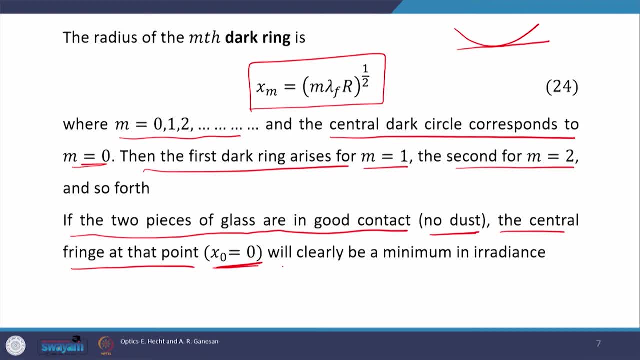 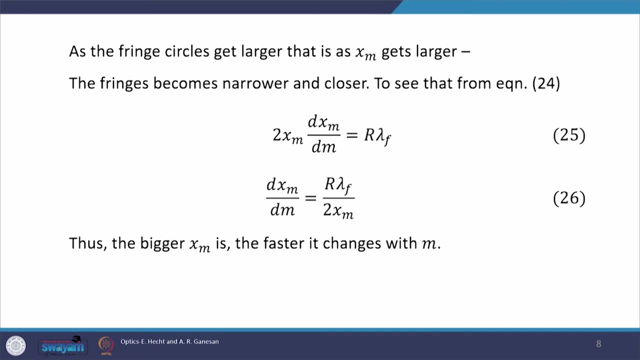 0th order fringe. it will clearly be a minima in irradiance here. You will not see any bright patch there. Okay, So this is the perfect dark. Now the second observation. what people have observed in case of Newton's ring is that 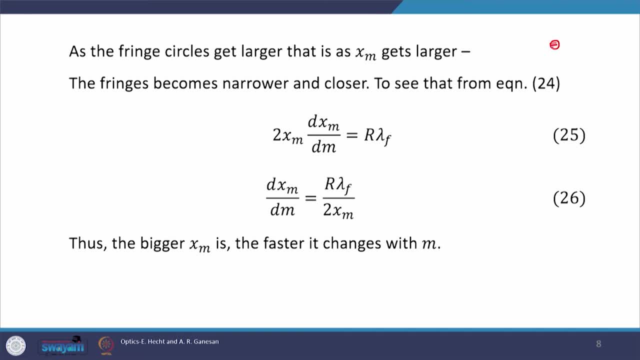 the centre is obviously dark- This we have understood- and then bright and then again dark. But if we keep drawing more circles, then what happens is that the circle is start to come closer as we move away and their width also reduces. Okay, If you go away from the centre, the width of these fringes reduces. 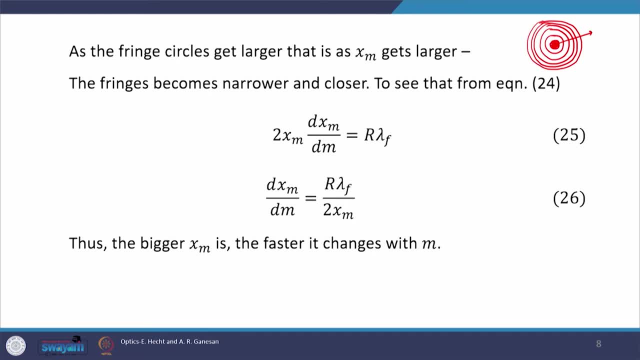 Okay, And this is observed in this case. Then the people start asking: like: what is the reason? Why does the fringes start to shrink if we move away readily outward? Okay, This can be understood from sorry, This can be understood. 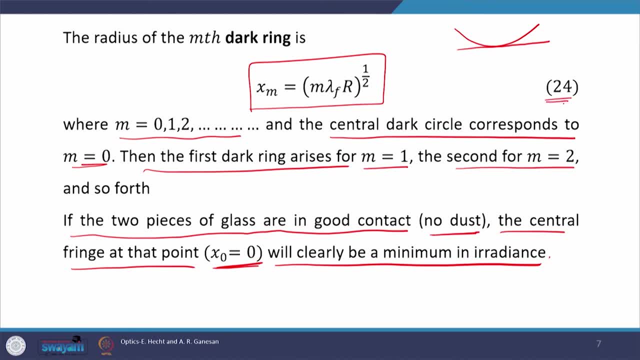 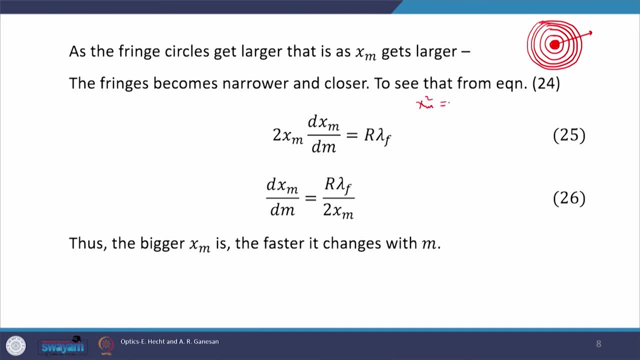 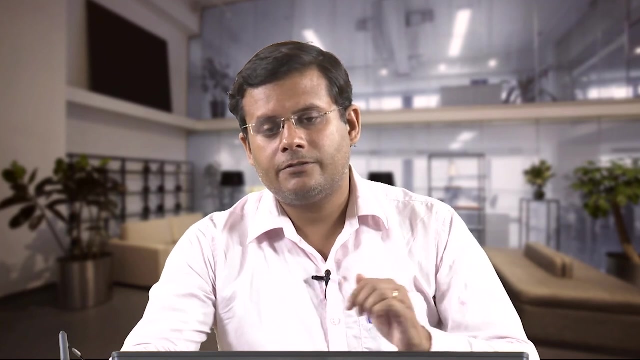 This can be understood from this equation, Equation number 24.. Okay, Equation number 24 can be written as xm square is equal to m lambda f into capital R. Okay, Now we want to see, or we want to observe, the variation in the radius of different fringes. 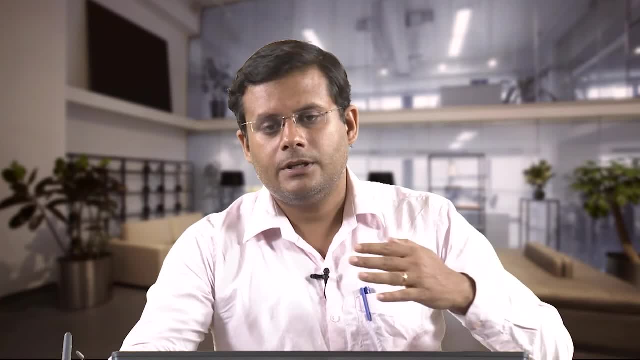 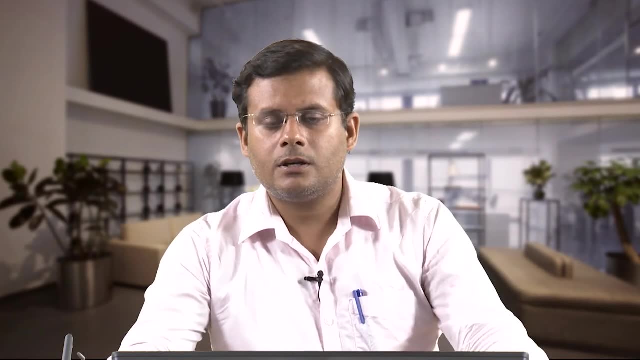 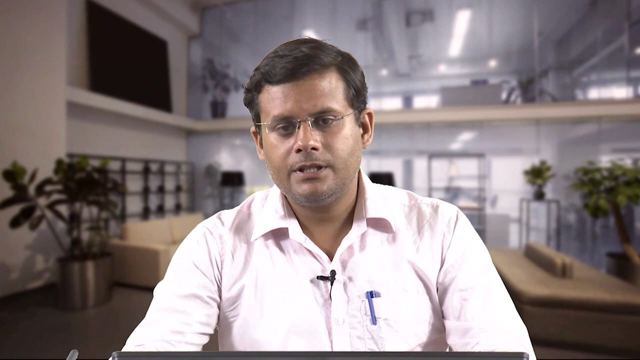 with respect to change in order. Okay, If we go readily outward, then the fringe width decreases. means if we increase the order of fringes, then fringe width is decreasing. Yeah, Or let me reframe it: If we increase the order of the fringe, then we see that the fringe width is decreasing. 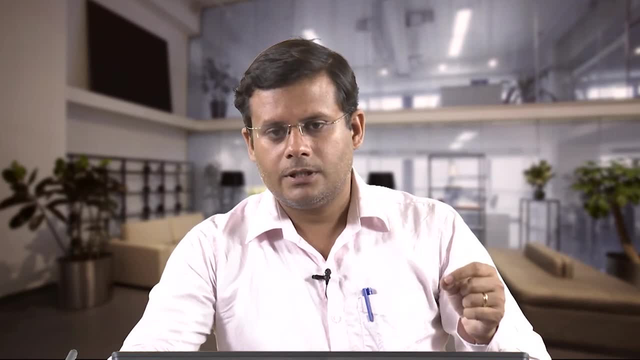 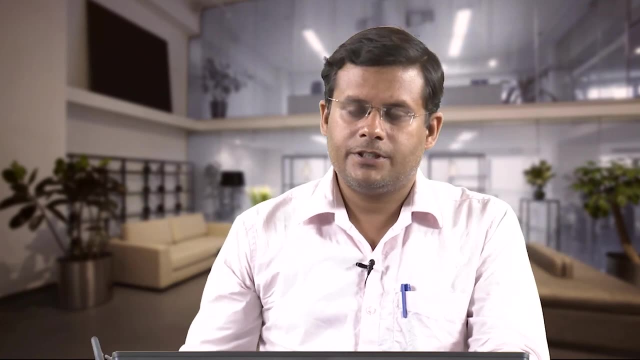 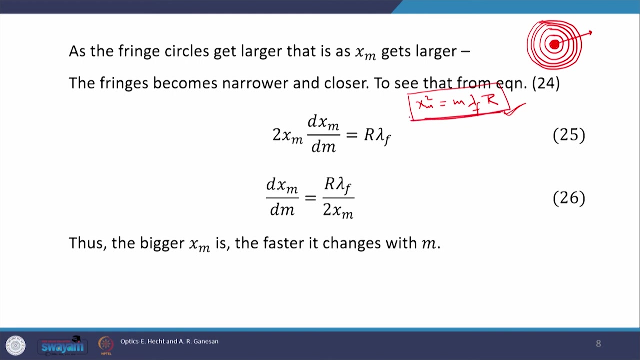 and this statement is similar to that- if we go readily outward, the fringe width decreases. Okay, Now, this decrease in the fringe Fringe width can be seen in this relation. this equation 24.. How, differentiated with respect to m? Now, if you differentiate this equation, then you get equation number 26.. 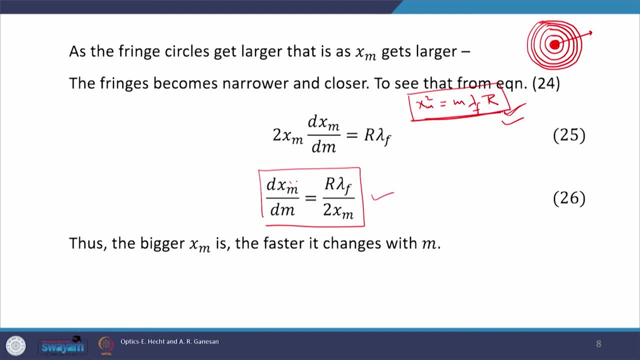 This represents variation in the radius of fringe with respect to fringe order. Now we see that this variation is inversely proportional to the fringe radius. Okay, Okay, Okay. It means, as the radius increases dxm by dm, which is the left-hand side, this becomes: 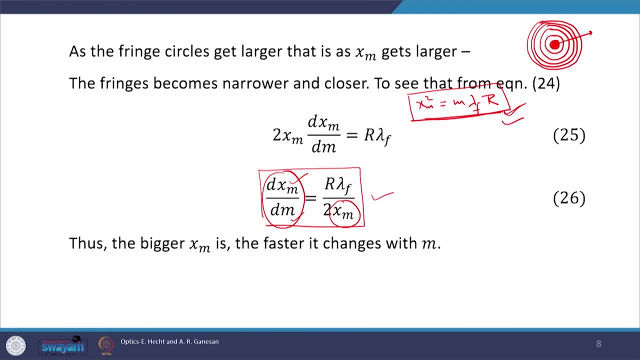 fast. Yeah, This is what it is written here. The bigger xm is, the faster it changes with m. Okay, And the equation number 26 exactly says it. Now We see that as we move away from the centre, the fringe start to shrink here. 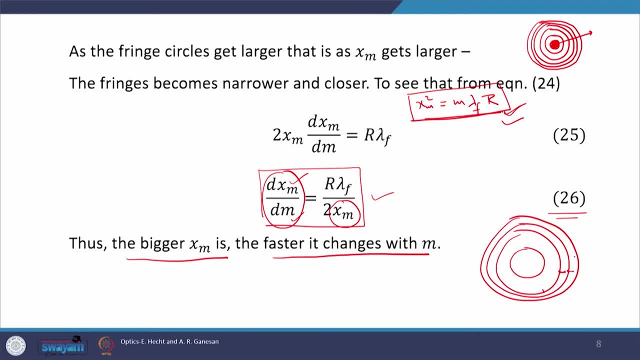 This: the fringe become closer and closer Now. but this can also be understood from the fact that this arrangement- this is the upper surface of glass. Okay, This is the convex land surface. This is not perfectly a linear wedge. The linear wedge is like this: 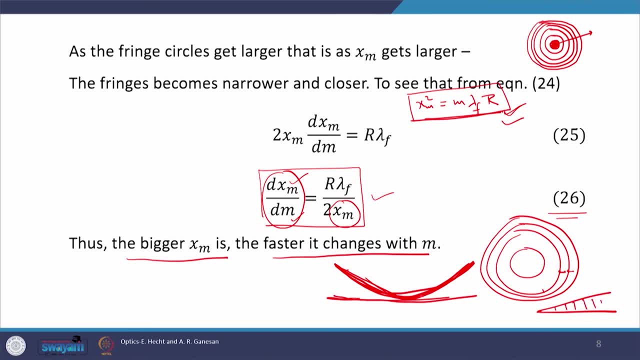 Okay, It is linearly increasing. But here you see, the surface is not a flat, here it is having some curvature. Okay, Now, due to this curvature, now, this air gap- let me pick a different colour. Now, air gap here is this much. 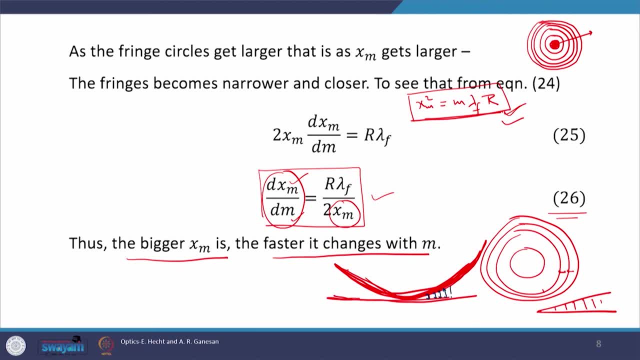 But as we move outward, the air gap quickly increases. Okay. Or alternatively, what we can see is that the condition of maxima and minima, the maxima goes to minima after lambda by 2 distance. Why? Because the second beam, second reflected ray, travels the this air width twice. 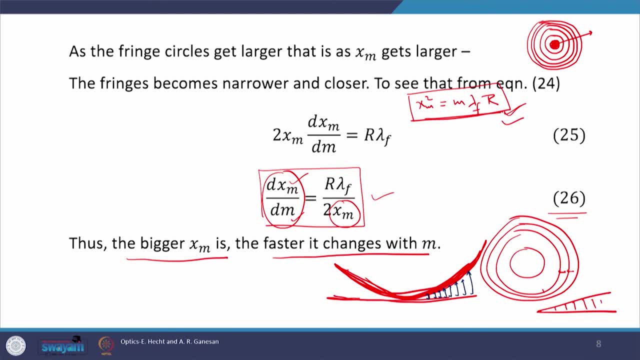 And therefore, As soon as there is an increase in the width by lambda 0, by 2, the dark fringe will go to bright or bright fringe will go to dark As we move away from the centre of this arrangement, the fringe thickness or the air gap thickness. 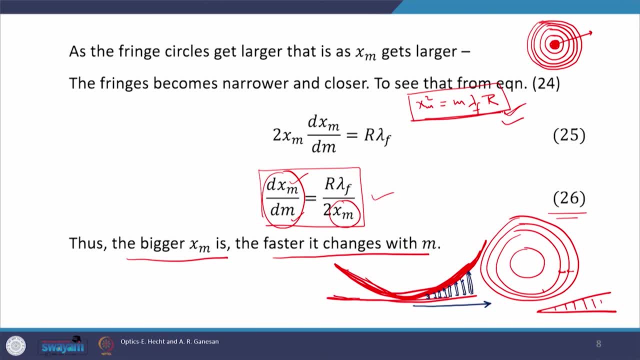 increases rapidly. Yeah, The fringe, the darker, dark fringe, goes to bright when there is a gap. Okay, So the air gap thickness increases rapidly. Yeah, So there is a difference in the air gap by lambda, by 2.. 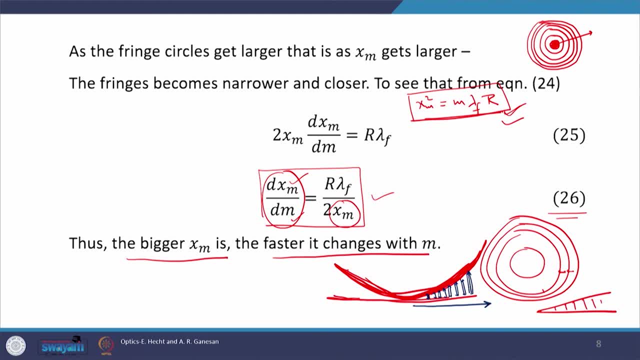 Okay, If air gap increases by lambda, by 2, the dark fringe changes from changes to bright one, or the bright fringe changes to darker one, dark one. This changeover happens rapidly here when we are far away from the centre, But this changeover is slow here. 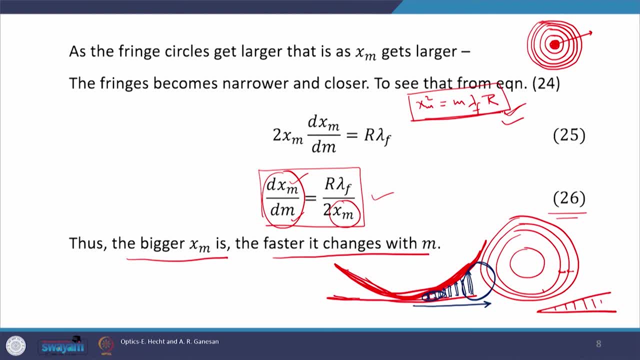 Okay, Because the width is increasing rapidly here. Okay, Since the width is changing rapidly here, therefore, the bright and dark fringes appears to be very close. Yeah, They become very thin, Okay, While when we are close to the centre, they are very wide. 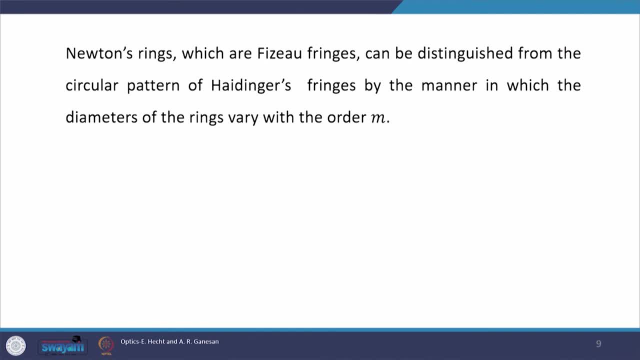 Okay, Newton's ring fringes. we know that the light is almost falling normally, and then we are getting concentric, circular fringe pattern. Therefore, this satisfies the condition. Therefore, this satisfies the criteria of being Faisal fringes. Okay, Therefore, these are Faisal fringes and they are different from Heidinger fringes. 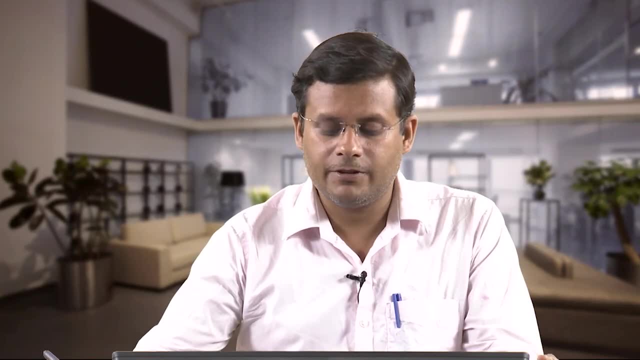 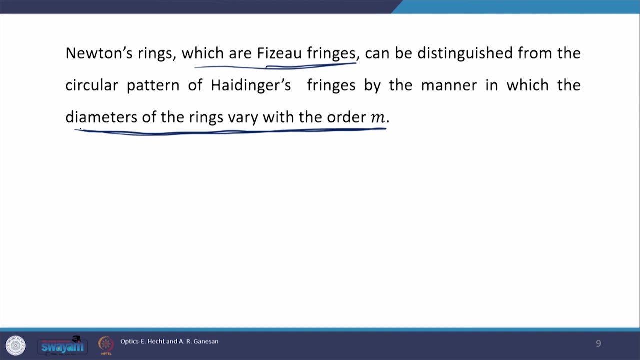 Okay, Faisal fringes are different from Heidinger fringes. What is the difference? The difference is that the diameter of the fringes. Okay, We know that both Faisal and Heidinger fringes are circular. Yeah, They both are circular. 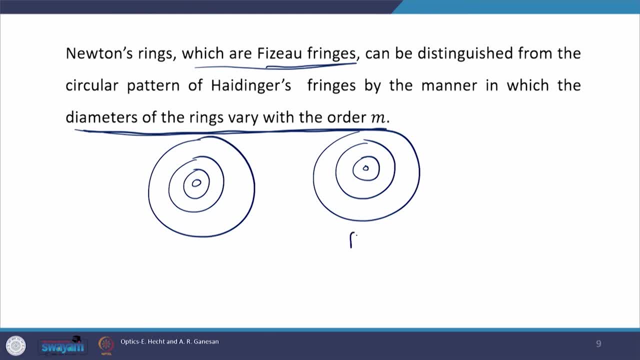 Okay, And this is say Heidinger, Heidinger. Okay, They both are circular. Just by looking at them, it would be difficult to distinguish between the two. They both are concentric circular fringes. Now, if you see the diameter of the rings, they vary differently with m. 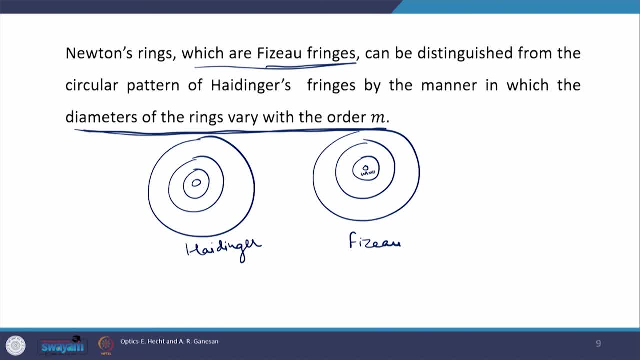 In case of Faisal fringes, m is 0 at the centre, and then if you move readily outward, then m increases. Here m is equal to 1.. Here m is equal to 2.. This is what also happens in case of Newton's ring experiment.